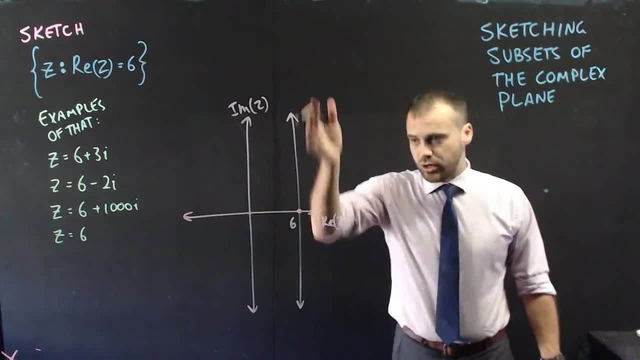 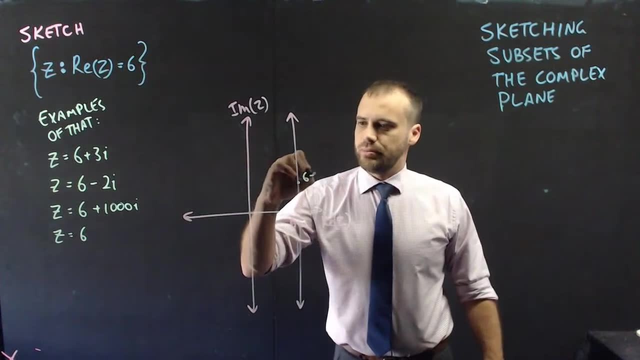 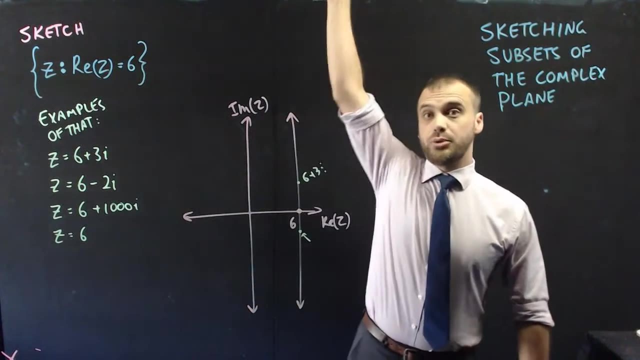 take forever. Instead, I can show it graphically On my Argand diagram. it's just a vertical line, right? Because 6 plus 3i would be like here: 6 plus 3i And 6 minus 2i would be down here somewhere And 6 plus 1000i would be way up here, And 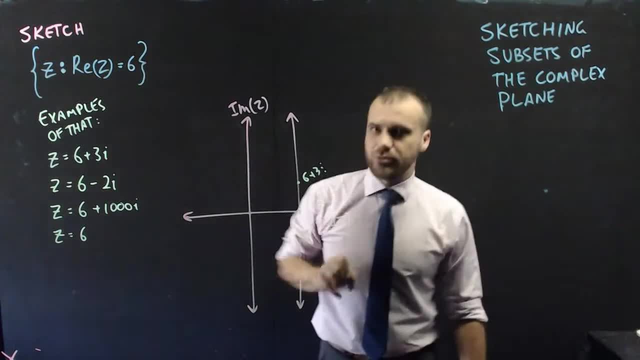 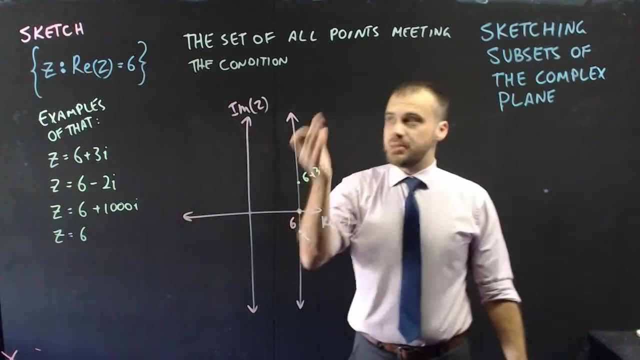 just plain old 6 or 6 plus 0i would be right there And we're showing all of them just by drawing in that line. Now we can say that this is the set of all points meeting the condition that's been set out, And this is sometimes called the locus. So if someone 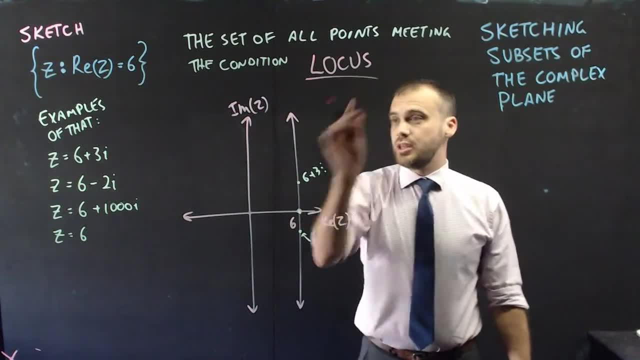 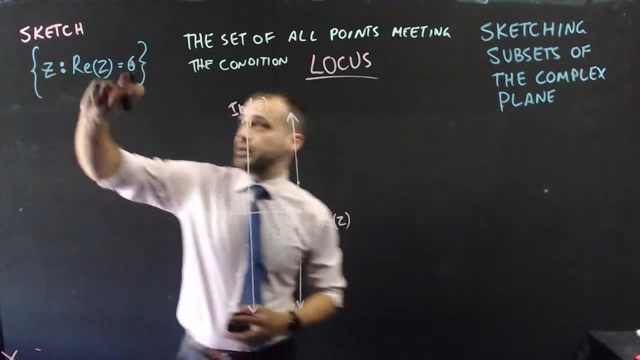 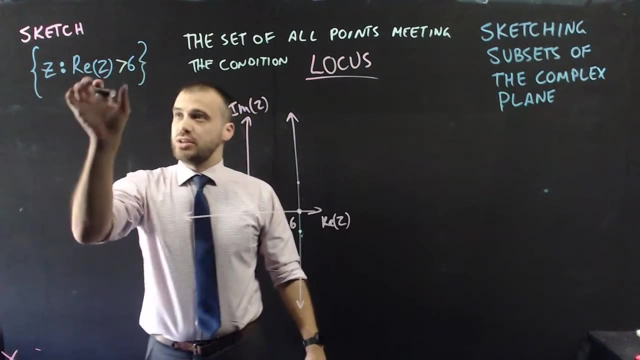 asks you to find the locus or sketch the locus. they're asking you to do something like this. Now I'm just going to change this question slightly and we'll see how the sketch changes slightly If we go from being equal to greater than it says the set of all z, such that their 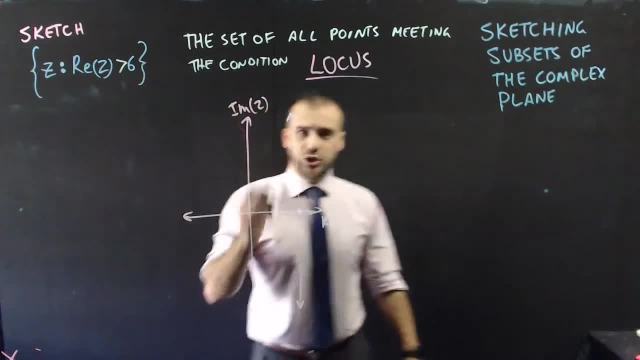 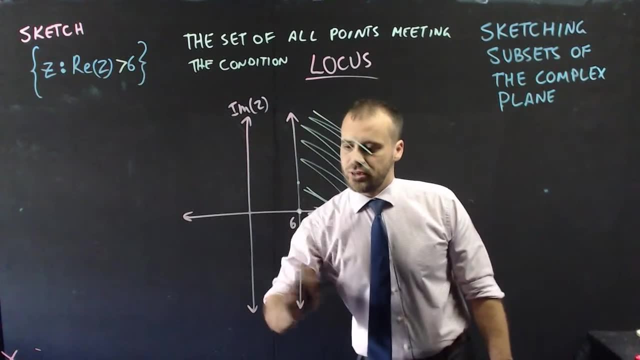 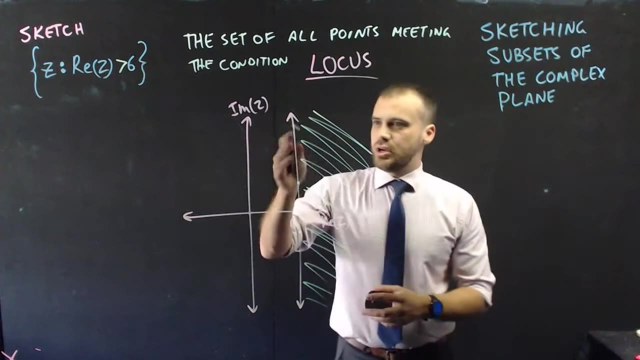 real components are greater than 6. And we can show that by doing two things. First, we would need to shade in this section here, right, These are all the complex numbers greater than 6. But this says greater than 6. So it 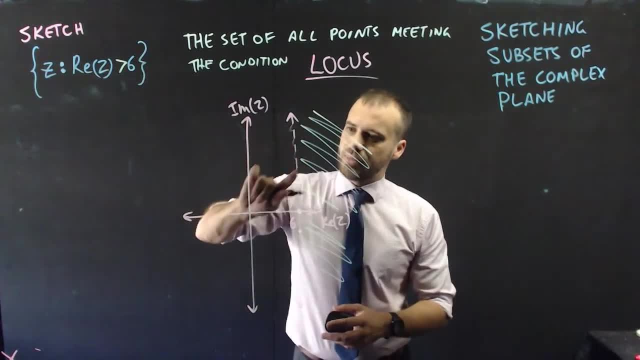 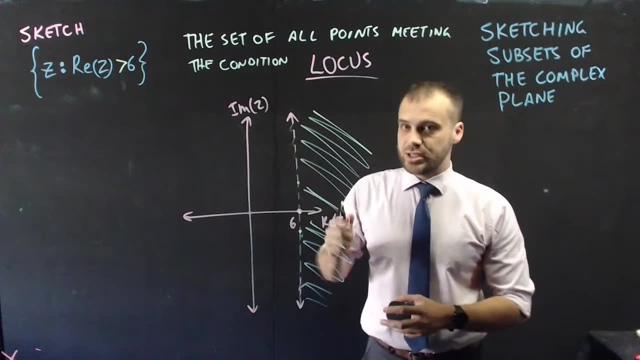 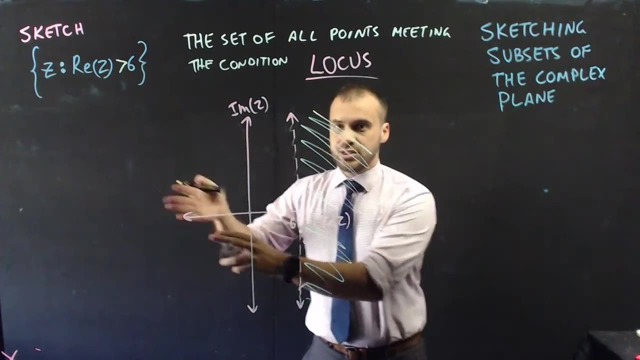 can't include this line. So we show that by making that line a dotted or dashed line. Okay So dashed line because it's greater than, and then greater than because it's on this side. If it was less than 6, obviously we would need to shade in this side. And if 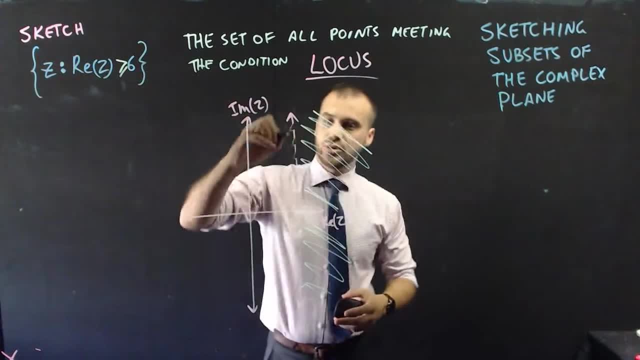 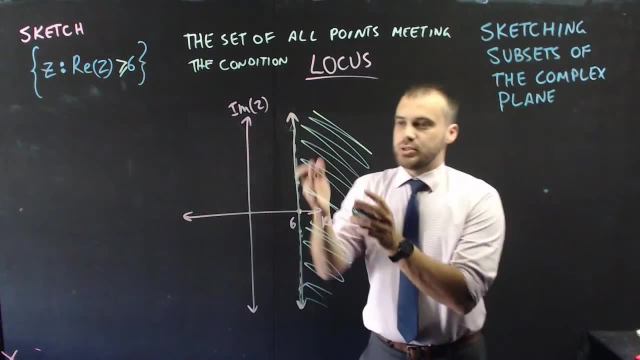 it was greater than or equal to, we would do exactly what we've done here, except our line needs to be solid Again, because it includes this line. All right, So a few different variations Now. the questions were never going to stay. 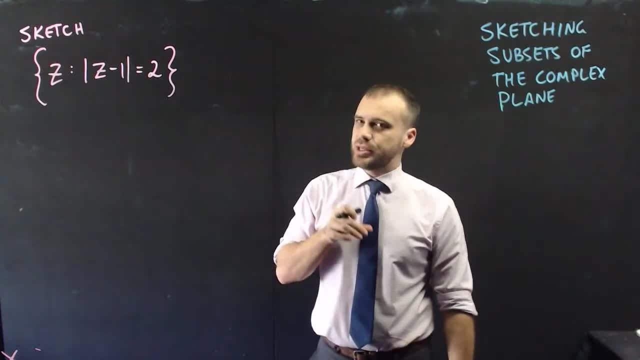 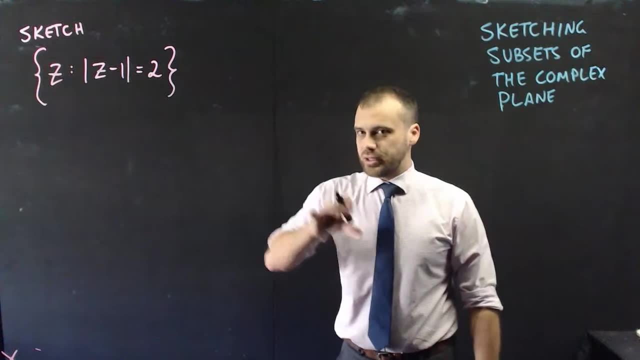 that simple. Here's a more complicated one, And there's two ways that we can tackle, and that's algebraically or geometrically. Now, normally I lean towards geometric interpretations, but algebraically, let's look at that one first, And what this says is the set of all. 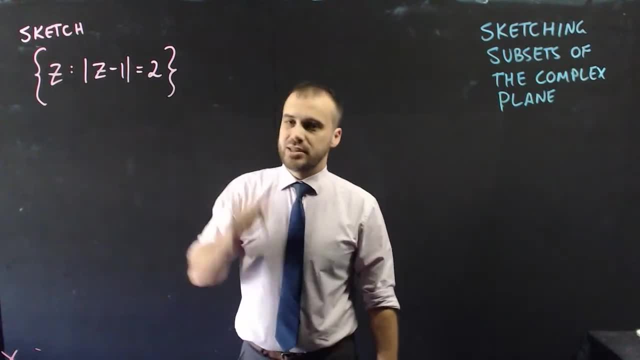 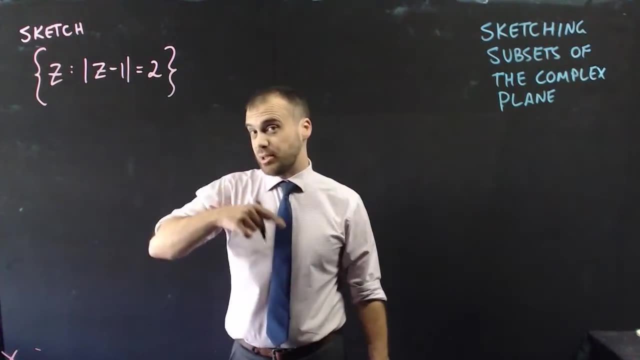 z, such that the magnitude of z minus 1 is equal to 2.. Now z is a complex number and that means that it can be expressed as x minus 1.. X plus yi, And when we do that we get our first line of working here: Magnitude x plus. 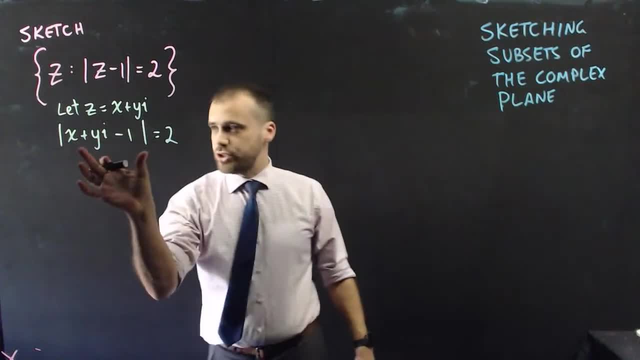 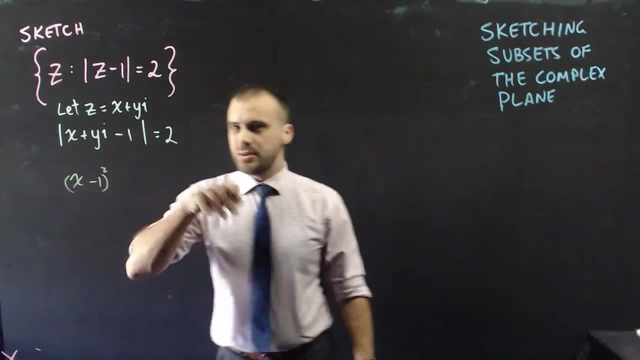 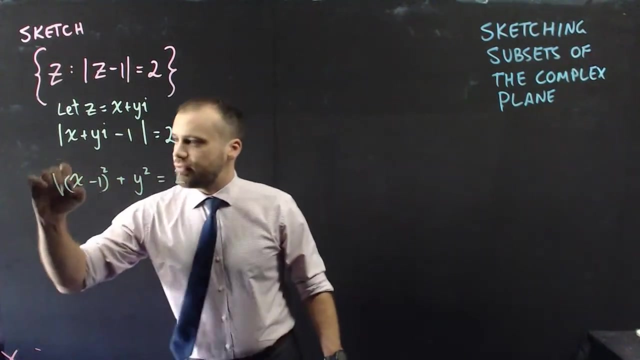 yi minus 1 equals 2.. Now we know how to find the magnitude of a complex number. We square the real components, which is x and minus 1, square the imaginary component, which is just y, and that's going to be equal to 2 if we square, root it right, We're just finding 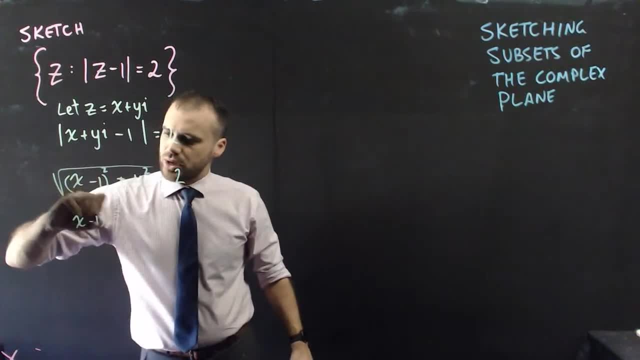 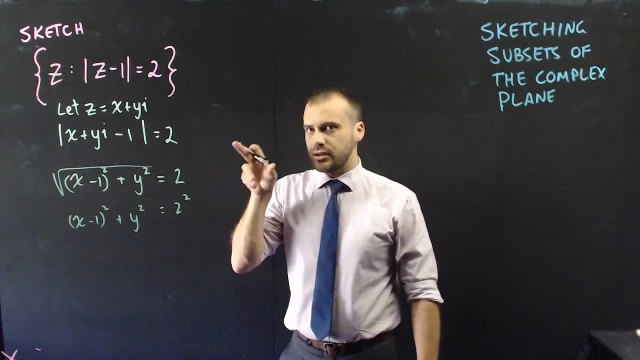 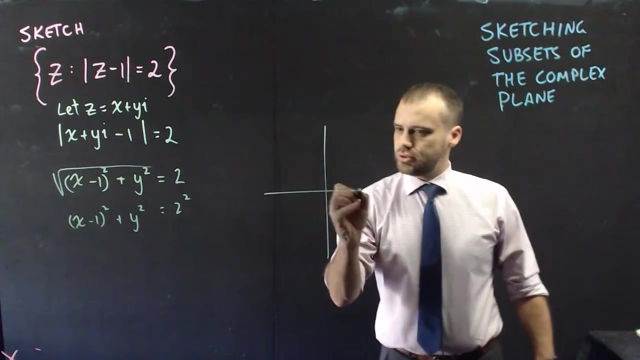 a distance. Okay, So what do we have? We have x minus 1.. Y squared plus y squared equals 2 squared. That looks familiar. We know what that looks like. That's a circle. That's a circle passing through this point here: 1.. Oh sorry, Having 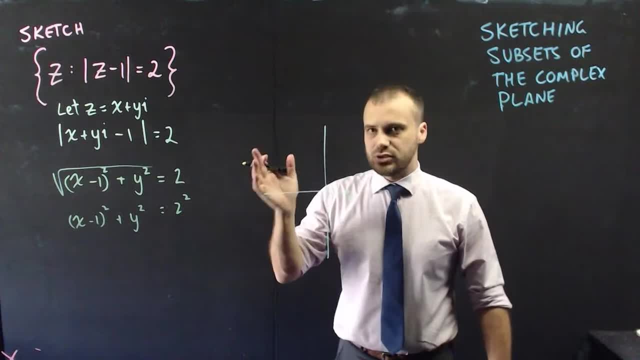 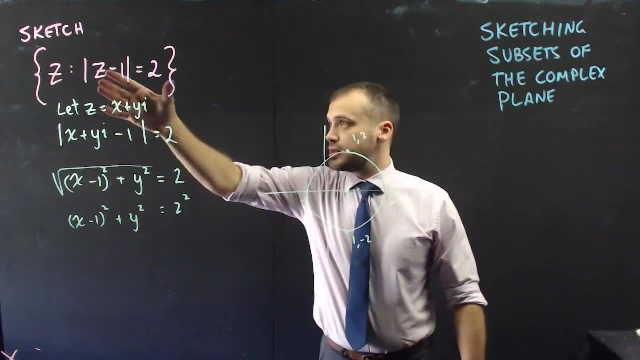 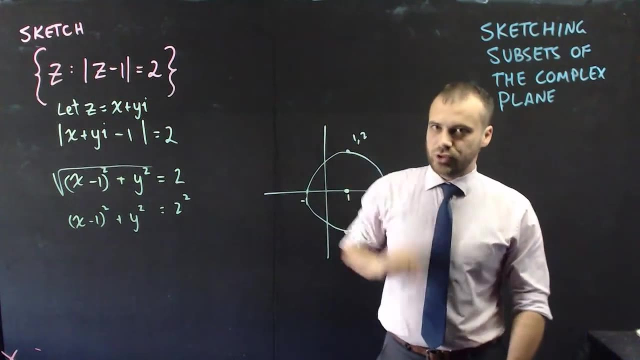 a center at 1 and a radius of 2.. And that's it. That's what I need. This circle here is the subset of Z that meets this condition. Okay, so I've worked through that algebraically and I've gotten that picture. You can also think about it geometrically, Okay, so what? 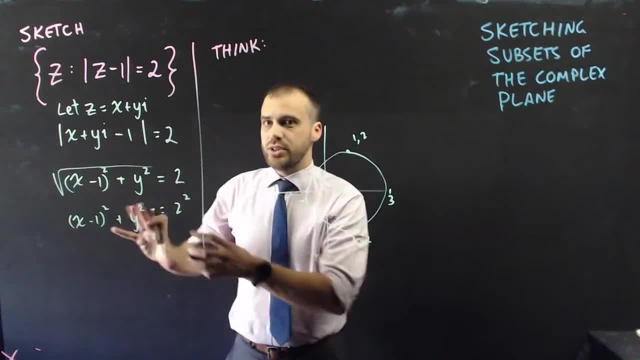 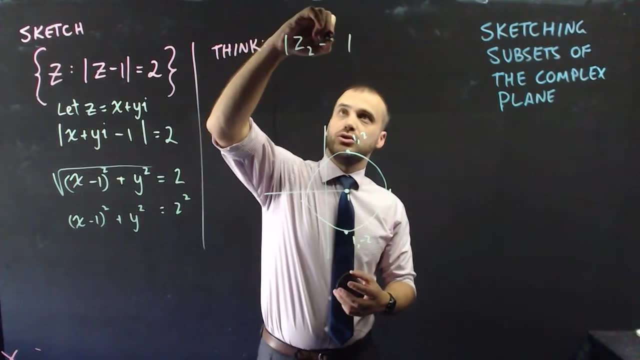 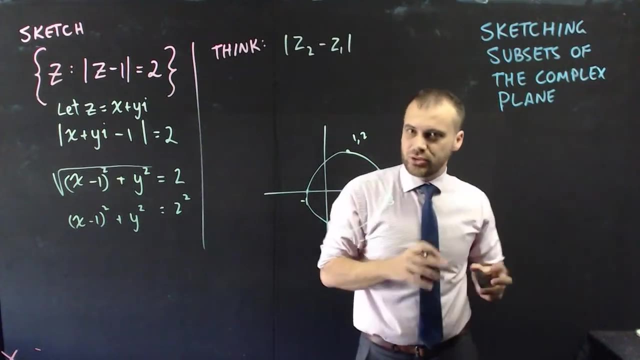 do I mean by think about it geometrically? Well, you can kind of avoid this working here and puzzle it out. So think, if I've got the magnitude between two complex numbers, that is the distance between their points on an Argand diagram, Okay, you can come up with. 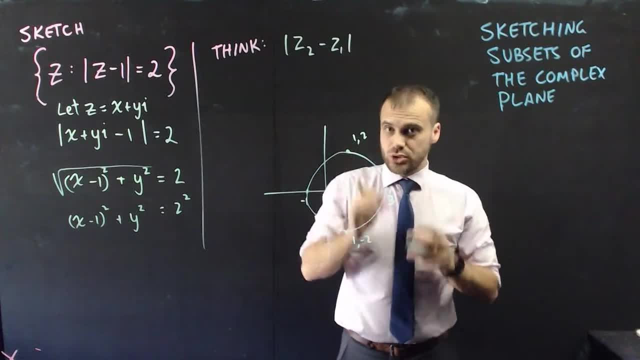 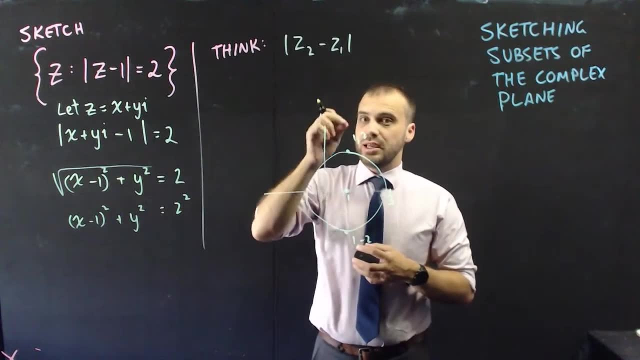 that You can figure that out. But that's what that is. It's the distance between two complex numbers. Now, in this one, we know what one of the complex numbers is. It's the number one, positive one, And you might be thinking, wait, negative one. No, no, no. 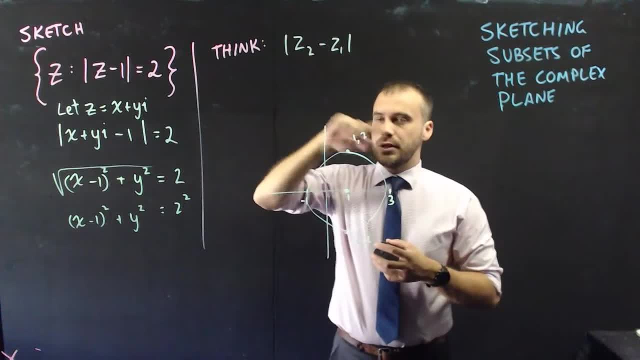 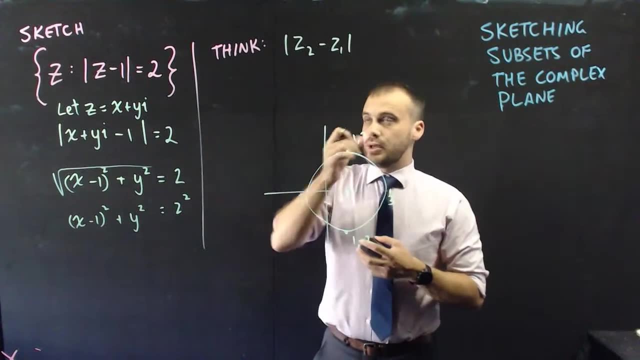 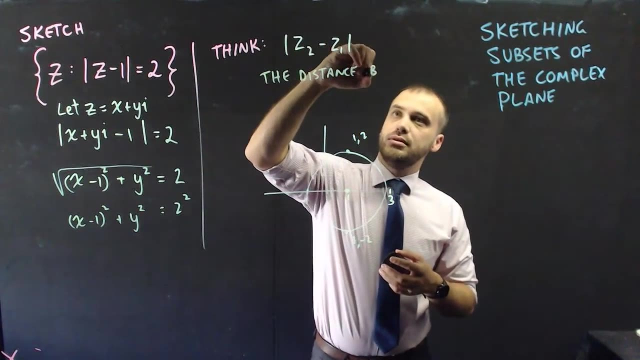 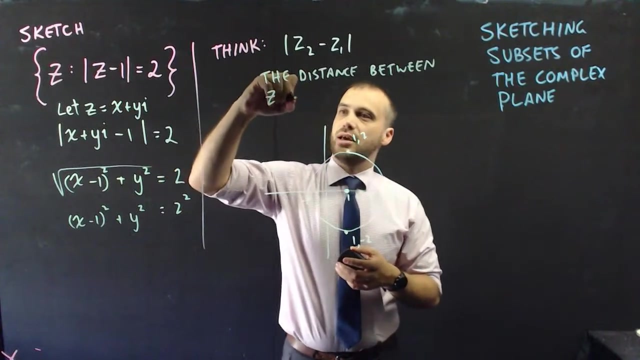 If we're subtracting two and finding the magnitude, then that's the distance between this bit here And that one, in this case, is positive one. Okay, so the distance between, in this case, whatever that was, Z and positive one because of what I just 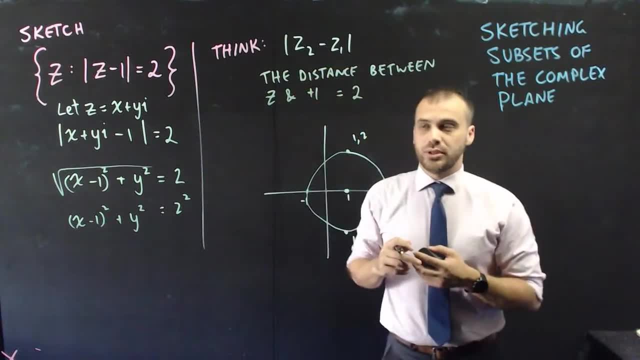 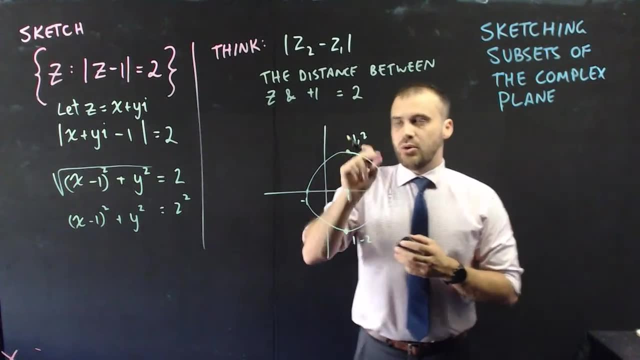 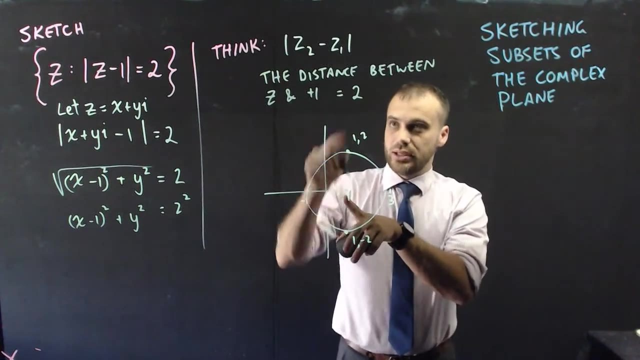 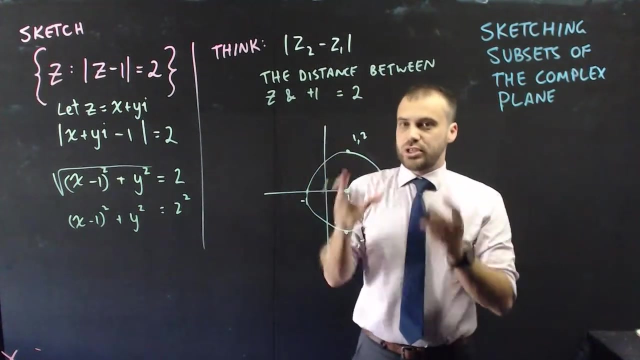 said, must be equal to two. Now, what do you get? if you're mapping all of the points on an Argand diagram where the distances between the point and just the number one is equal to two, You get a circle. Okay, that's the geometric interpretation. 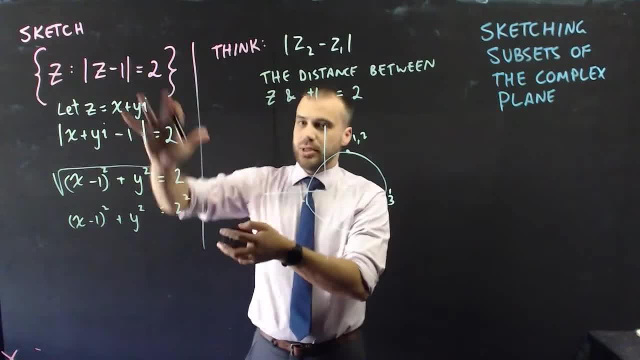 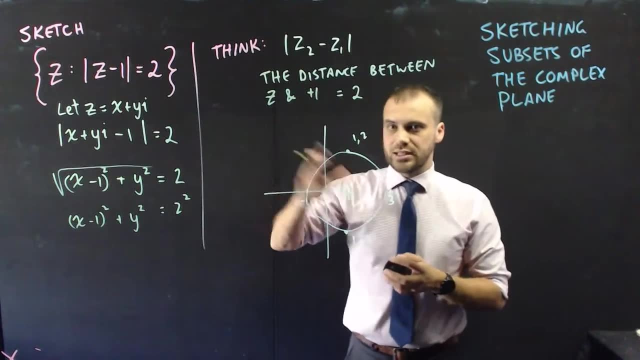 of it. I really think that this is probably a better way of working and then sketching whatever drawing you have. But if you can think in two ways, obviously you can check your answer against itself. Now I must say that there are a few variations of this question. 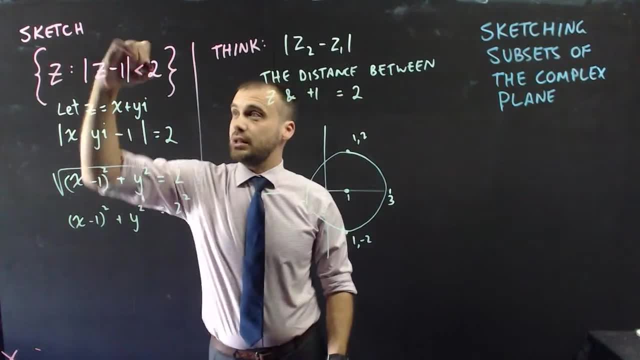 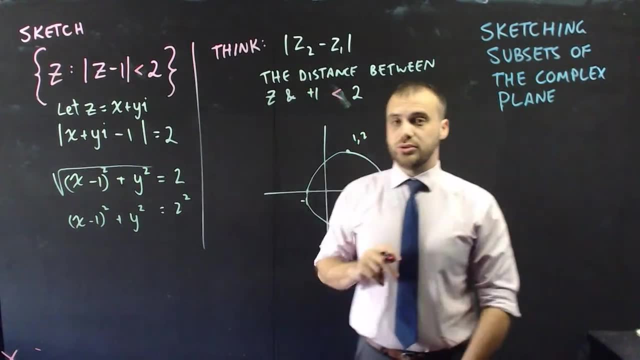 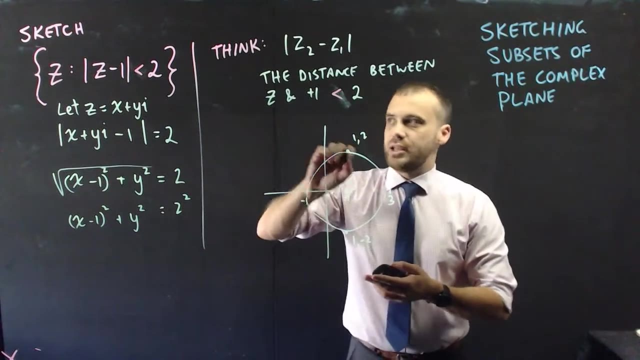 So it could be not equal to, it could be less than, And that means the distance between Z and positive one is less than two, And if the distance is less than two, that means we're inside the circle, Alright. And because it's 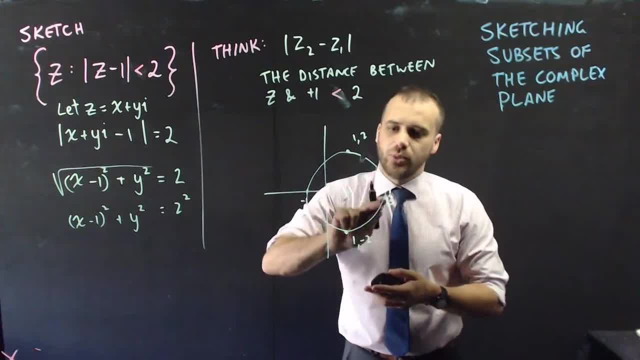 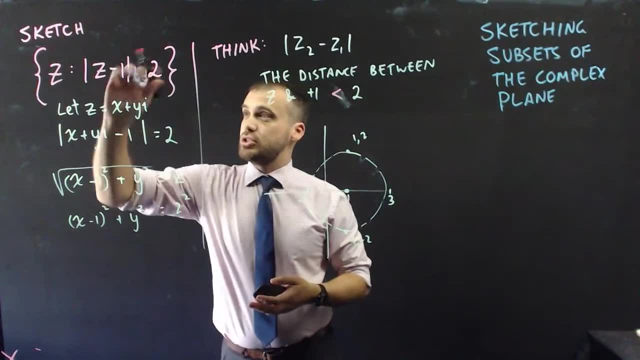 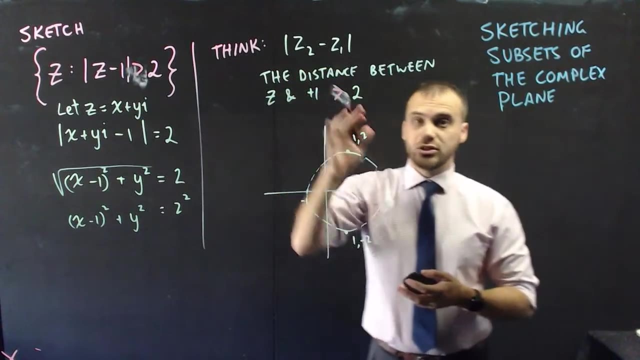 less than the circle wouldn't look like that. The circle would be a dotted circle because it's not including the circle. If I move this sign and turn it around, we're saying the Z is greater than two, And if that were the case, we'd be sketching outside of the circle. 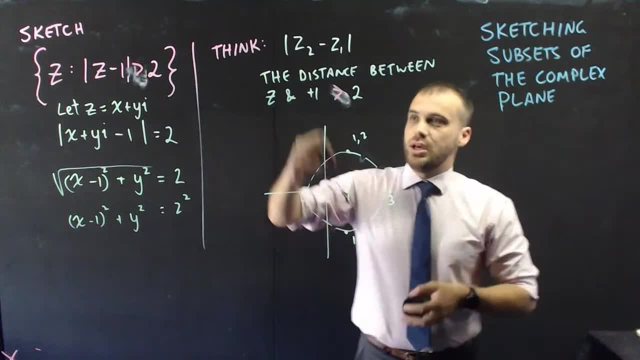 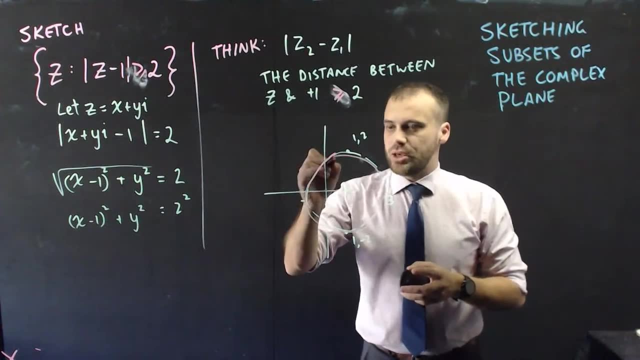 And again we would have this dotted line because it's greater than, not equal to. If it was greater than and equal to, we'd be sketching outside of the circle and our circle would be whole again. Now we can continue on here. This looks pretty intimidating. The. 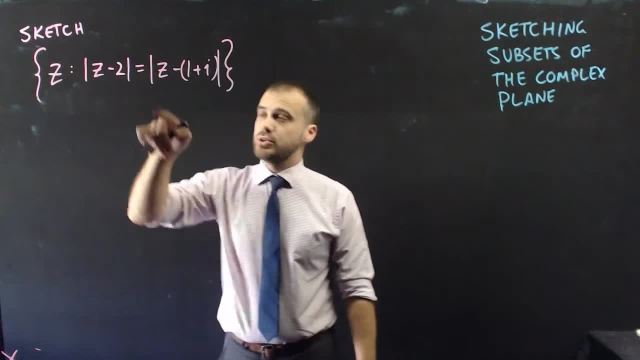 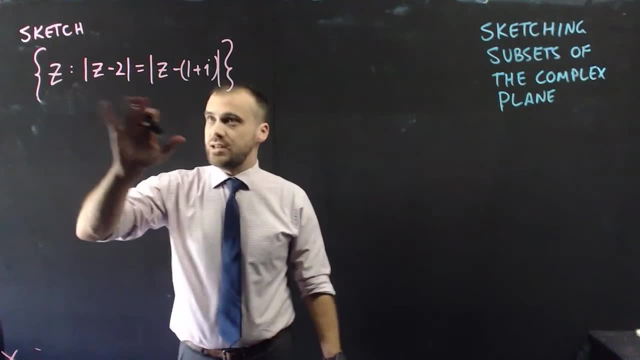 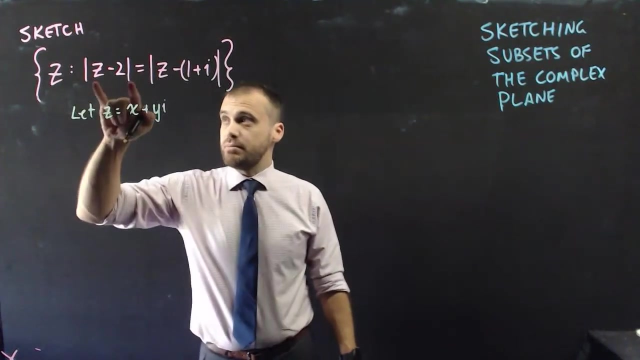 set of all Z, such that the magnitude of Z minus two is equal to the magnitude of Z minus one plus I. Now again, we can do this algebraically by understanding that Z and Z, they're the same Z. there We can express those as X plus YI, And once we've done that, we can find the. 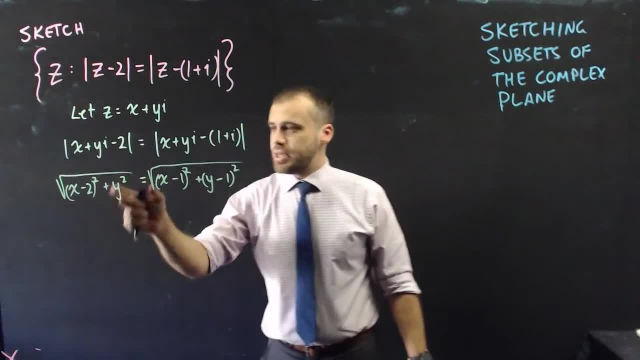 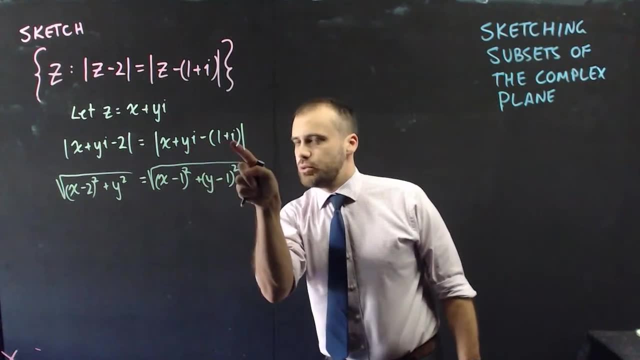 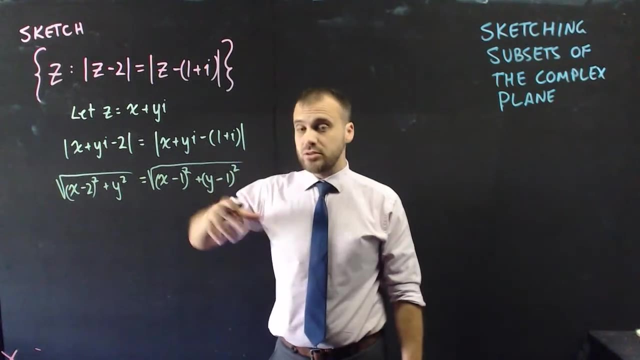 magnitude of this and the magnitude of that. So we've got magnitudes here. Be careful. I just had to group real components. I had to group imaginary components here, Y minus one, one, I, which is one. Alright, I can square both sides now, and then I can sort of expand. 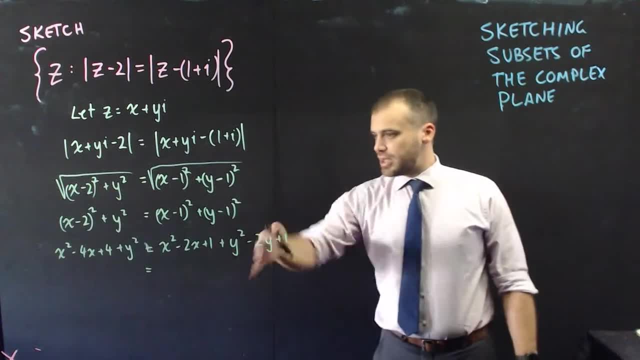 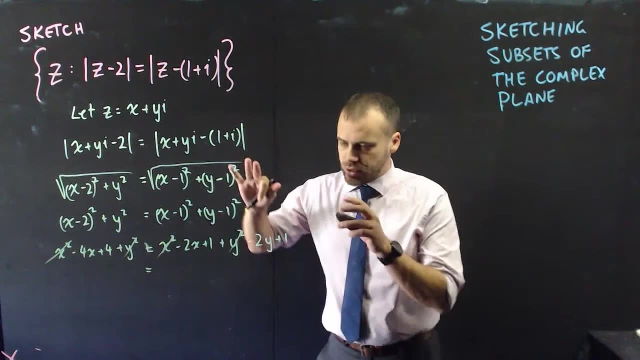 group-like terms, etc. etc. So once we've done that, we can get rid of some stuff. We can see X squared, X squared, Y squared, Y squared, And then we can narrow this down and see where we end up And we 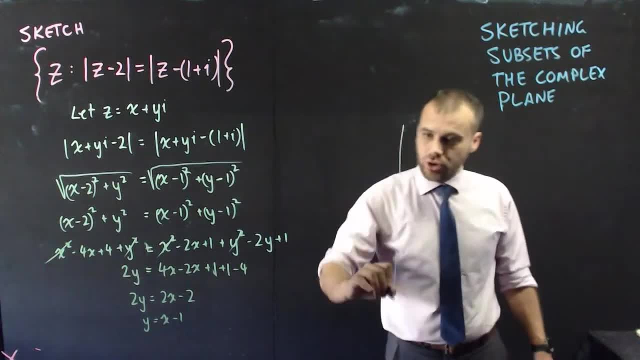 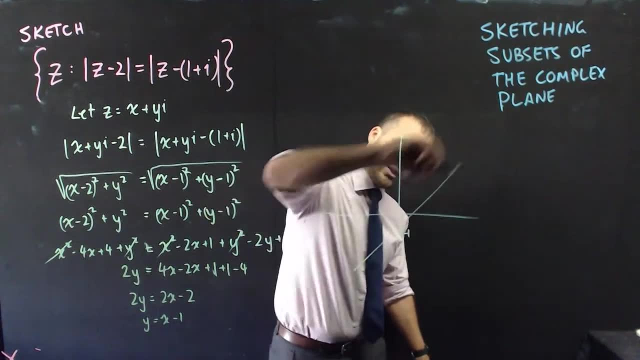 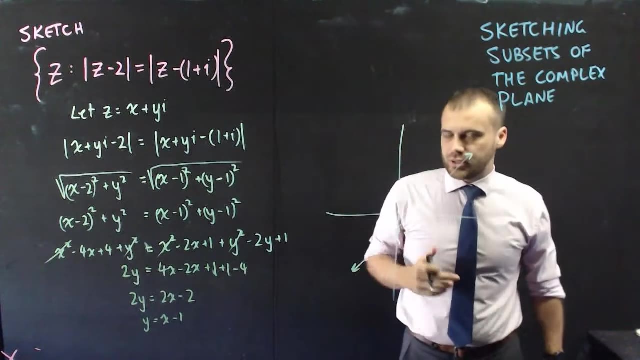 eventually end up at Y equals X minus one, which, on an Argand diagram, it's going to be pretty obvious. We're going to have here negative one. We're going to have a linear equation with a gradient of one, and things lying on that line are going to be our answer. 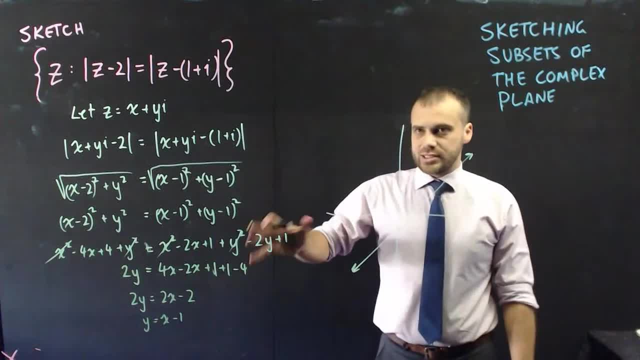 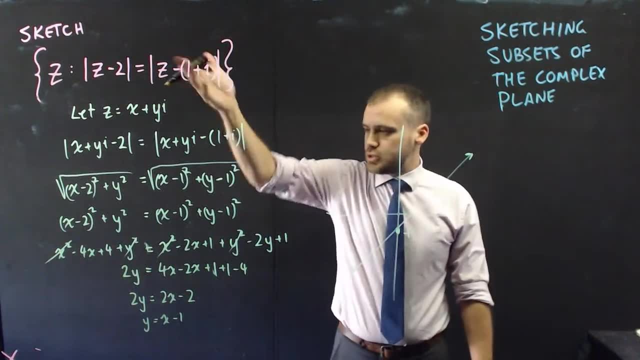 Now I'll leave you to figure out the greater than or less thans, if it was here or if it was the other way, But you can see that it starts off pretty intimidating, but once you start working through it, algebraically, no problems. 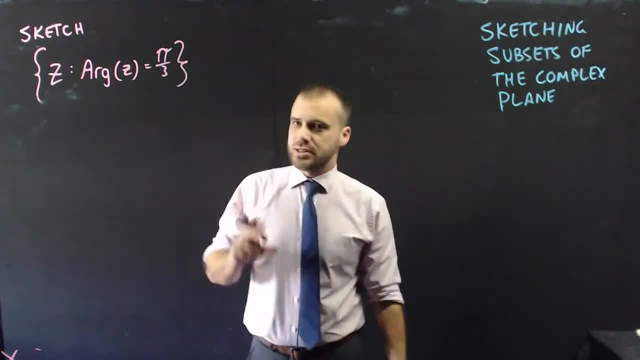 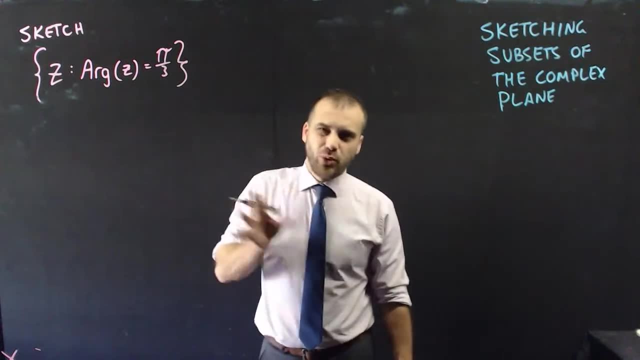 Next up we're going to look at a few different versions of this where the argument has some sort of condition. So this says that ArgZ is equal to pi on three. So here I'm not going to work algebraically, here We're just going to think geometrically. What does it? 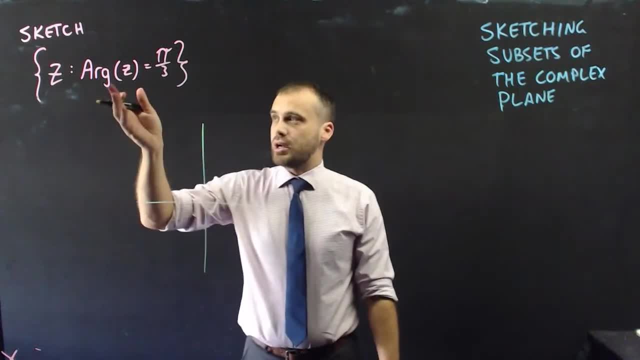 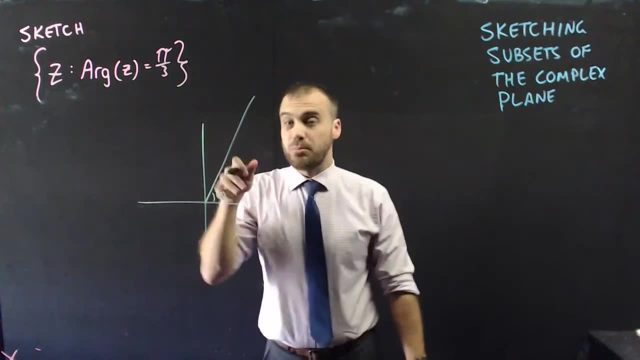 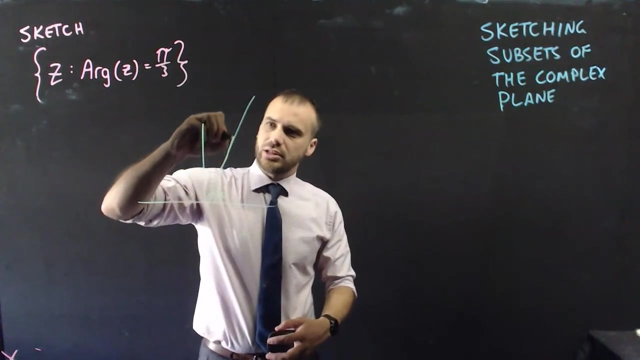 mean It's a complex number to have an argument of pi on three. It means that it makes an angle of 60 degrees or pi on three with the real axis. So anything lying on this line here has an argument of pi on three, and I've sketched it. 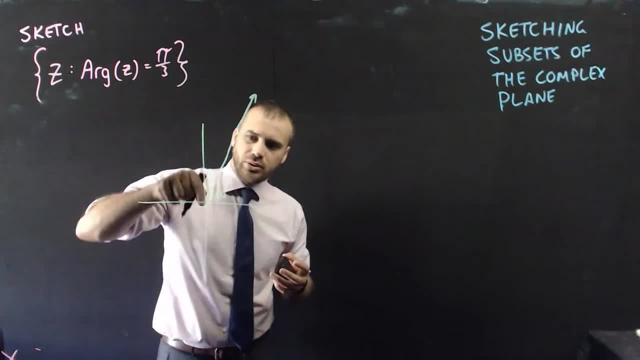 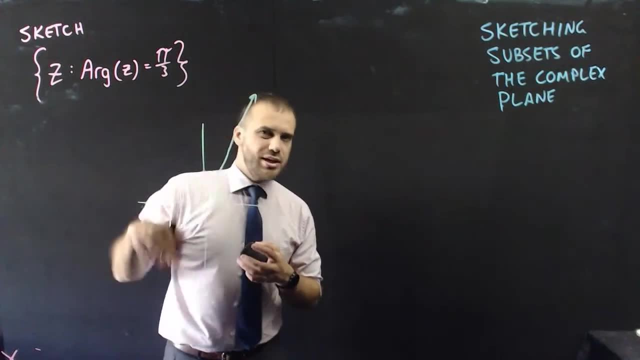 Now you might be thinking: but what about going down in this direction? Well, things in that direction don't have an argument of pi on three. They have an argument of negative pi on three. so they're not it. Alright, that's fairly straightforward. Let's look at another similar one Now. this is: 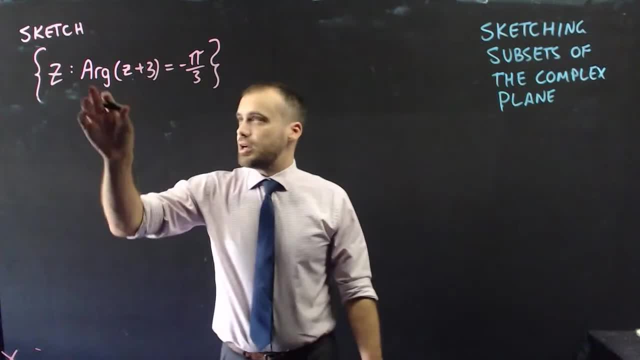 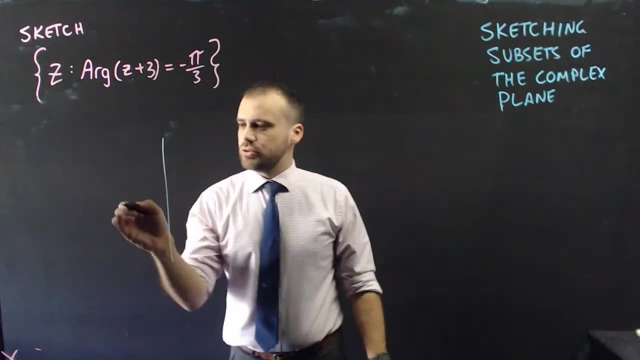 another one where you're going to want to think geometrically, The argument of a complex number plus three is equal to negative pi on three. Well, first of all, just forget the plus three for a minute. If it was just the argument of a complex number equals negative. 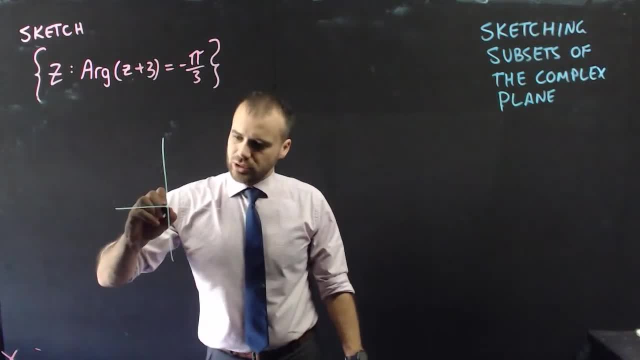 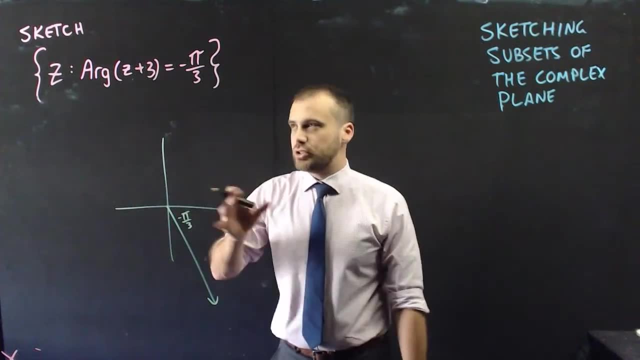 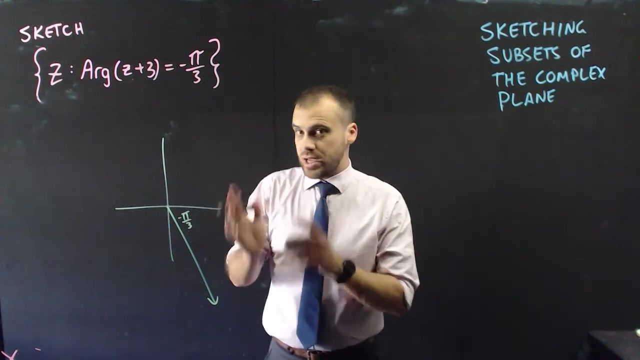 pi on three. well, that's pretty straightforward. We just lie on this line here, because that's the angle here is negative pi on three. But it's not just the argument of z equals negative pi on three, It's the argument of z plus three. Now we do the same thing that we do when 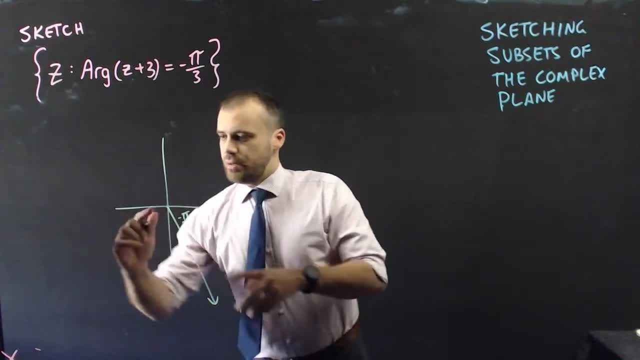 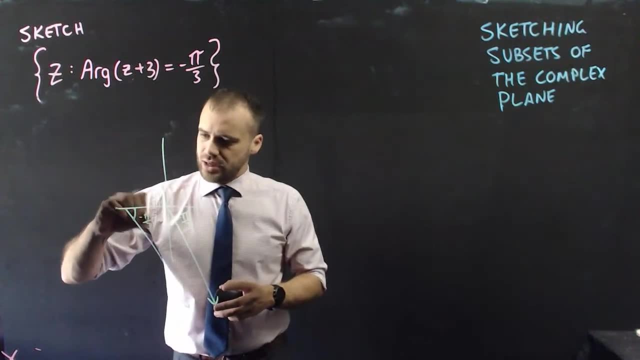 we're saying like plus three on any function, We're going to take that and move it three across. They're supposed to be parallel. Alright, that's negative pi on three there. This point here is negative three and any complex numbers lying on that. 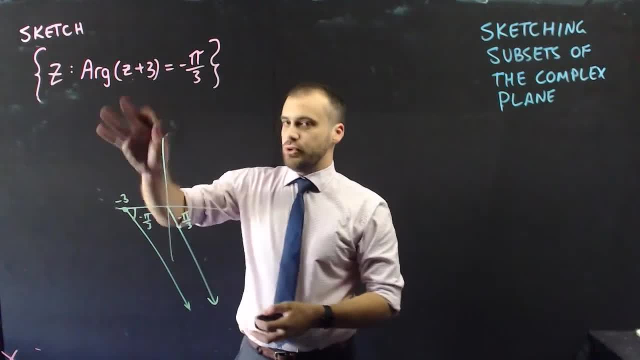 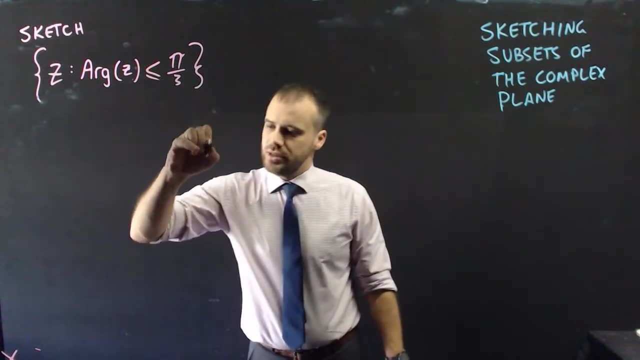 are filling this condition. This is our locus for this condition. Now this inequality is really worth exploring. so let's pretend it's an equal sign for a second. If it was an equal sign for a second, we're looking for all the complex numbers with an argument. 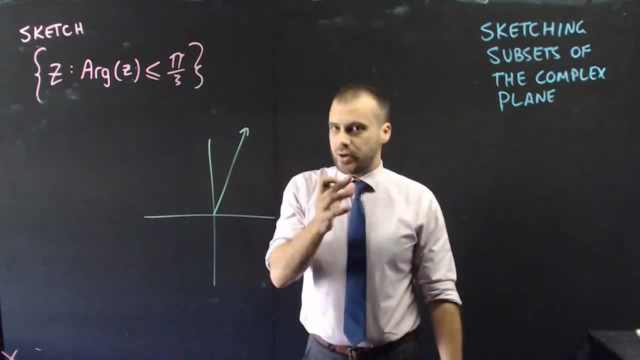 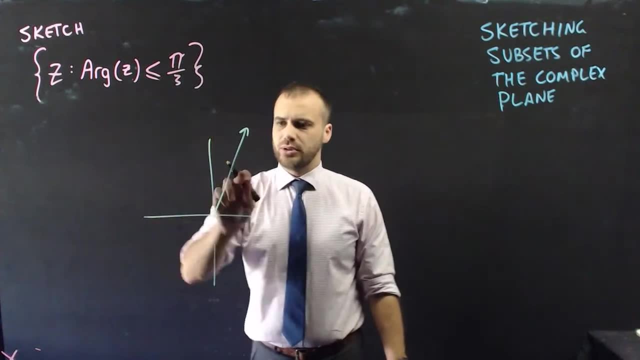 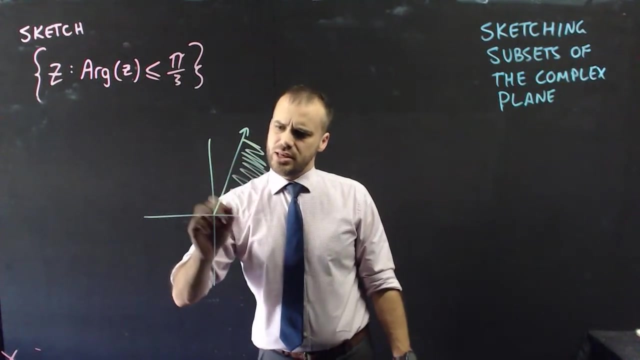 of pi on three. Okay, Now let's think What complex numbers have an argument less than pi on three. Well, there's probably one here, right? Because instead of being pi on three, it's less than pi on three. So anything in here has an argument less than pi on three. 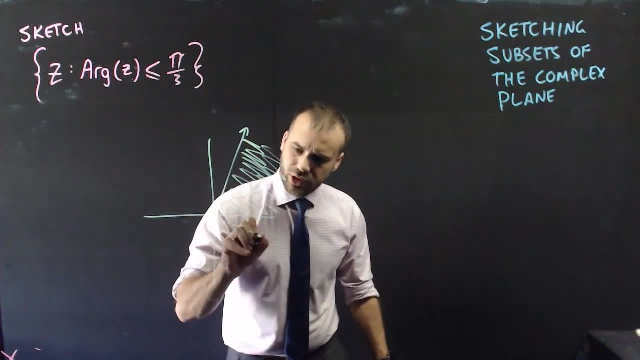 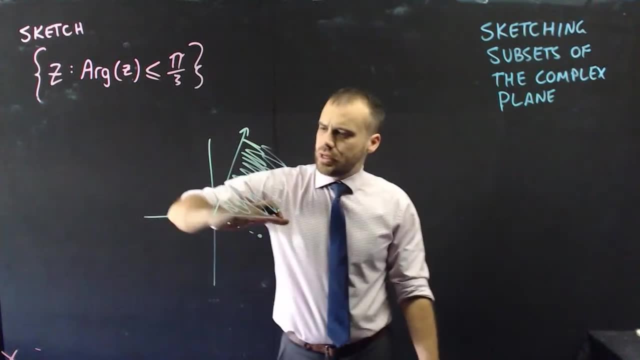 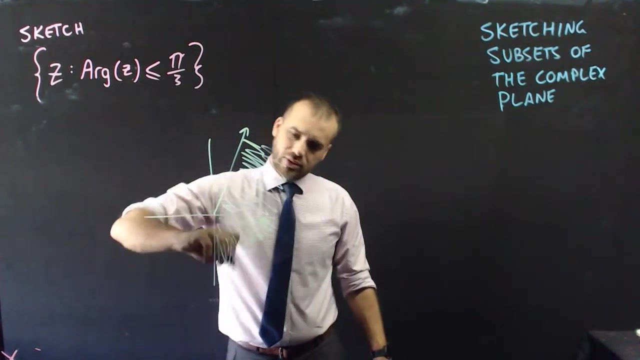 But if a complex number were here, say, right here, that argument is negative. negative let's talk in degrees negative. 20 degrees Negative is less than pi on three. so yes, this would be included as well. Now all negative arguments are all here, like this: 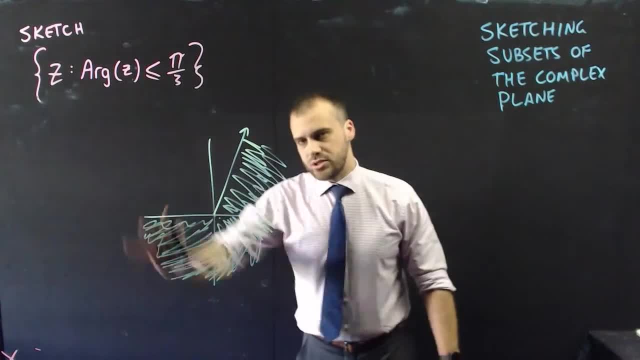 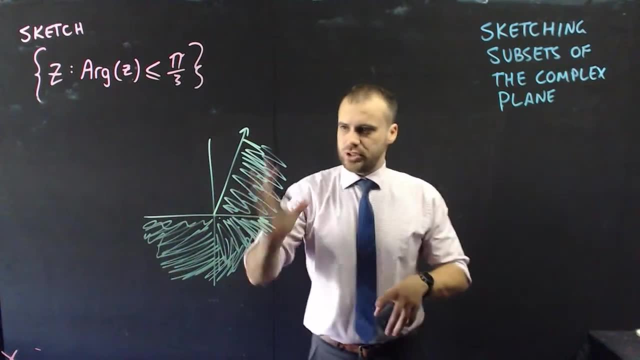 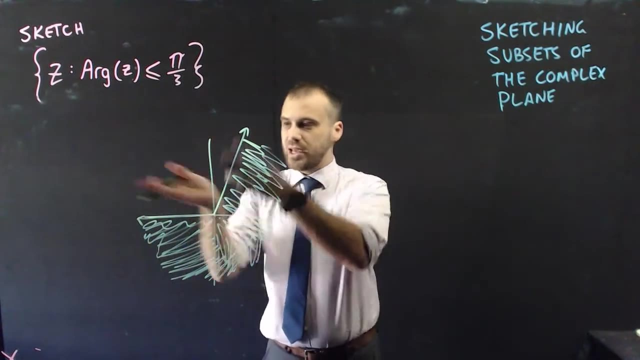 and so you end up with this strange sketch where it's all of that and then all the way around, forever and ever and ever in that direction, forever and ever and ever in that direction. it's just this wedge of our circle, of our circle or of our plane, that's not colored in so less than 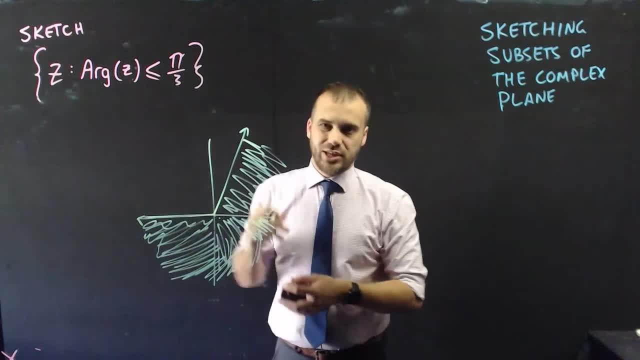 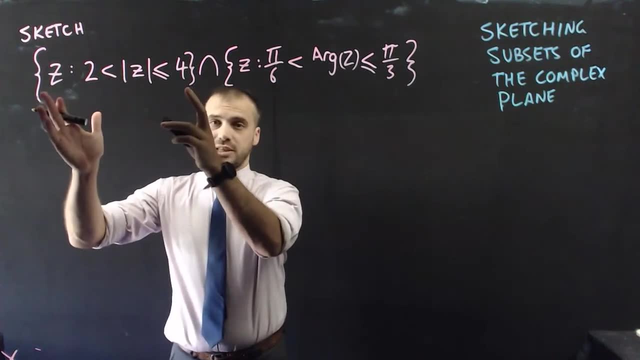 or equal to pi on three. i can keep that solid because it's a less than or an equal to one last one, saving the best for last. here, what we have is a set of conditions that need to be met and another set of conditions that need to be met. so we need to consider this. we need to consider 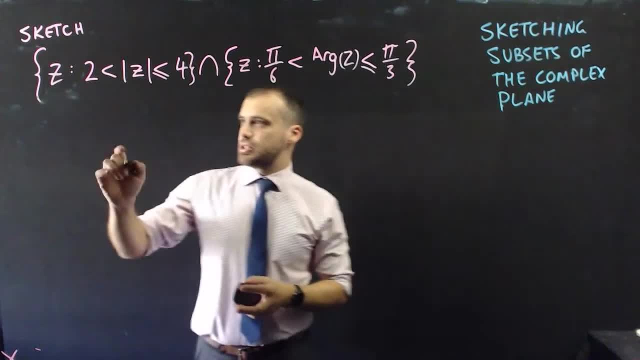 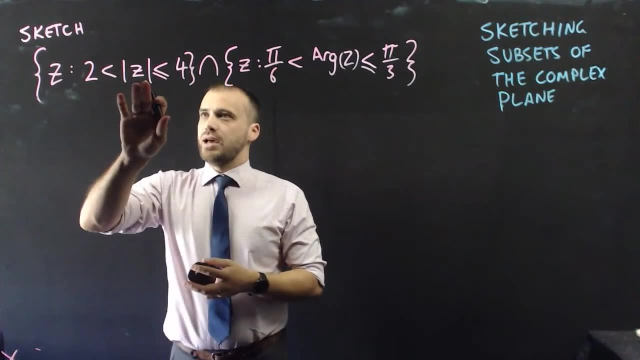 this and we need to consider where they overlap. all right, so let's look at this one first. this says: um, this condition here says that the complex number has to have a magnitude between two and four. all right, so if a complex number has a magnitude between two and four, it's going to 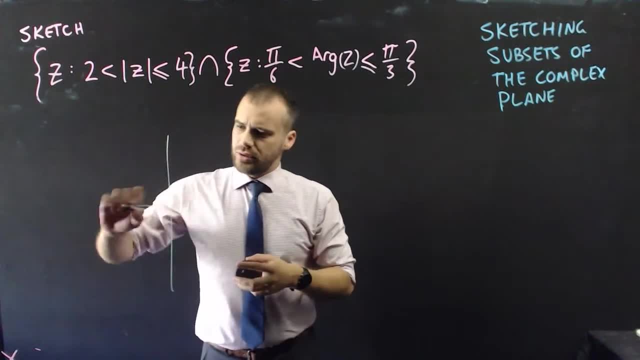 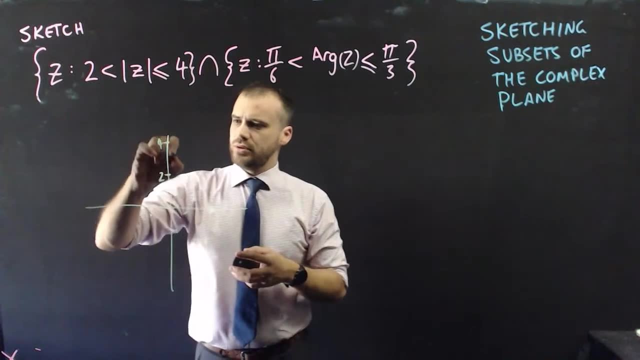 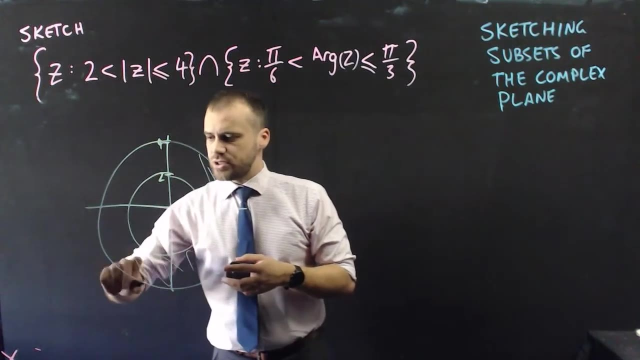 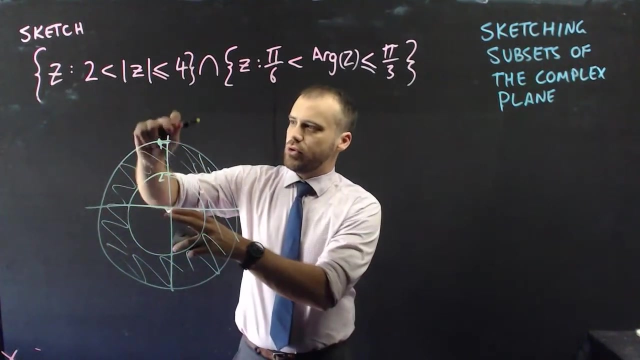 have a magnitude between two and four. that means that it's two- four. it's in this region of a circle, okay. so length of two: no. length more than four: no, can't be that either. so it needs to be between these two. now there's some complications here. 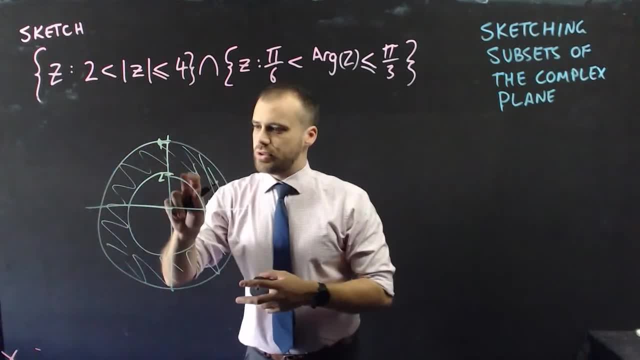 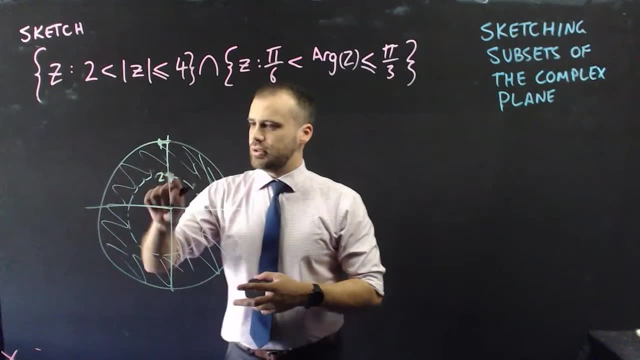 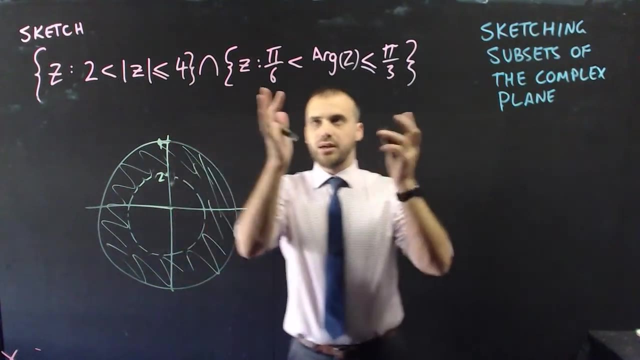 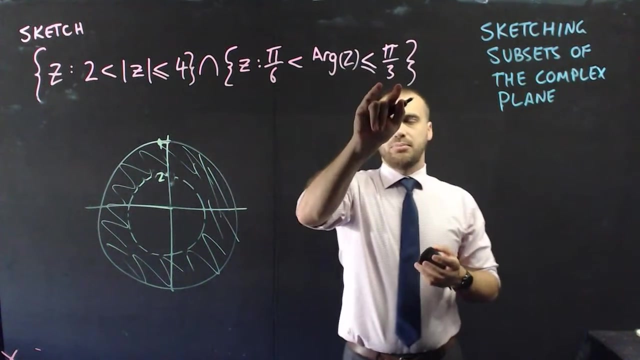 it says, uh, less than all right. so this needs to be a dotted circle here, because that one's not included, all right. but this one is, a is a defined circle because it is included. okay, what about our other one? uh, z needs to be, or argument of z needs to be, between pi on six and pi on three. 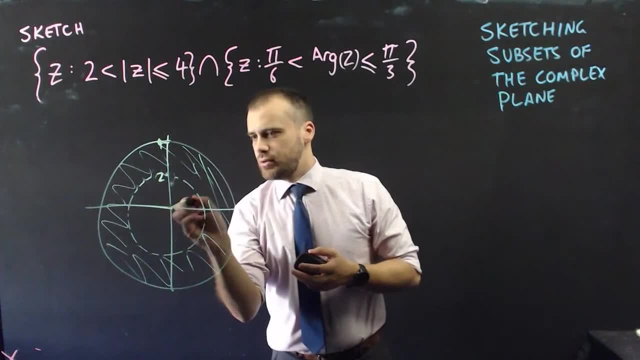 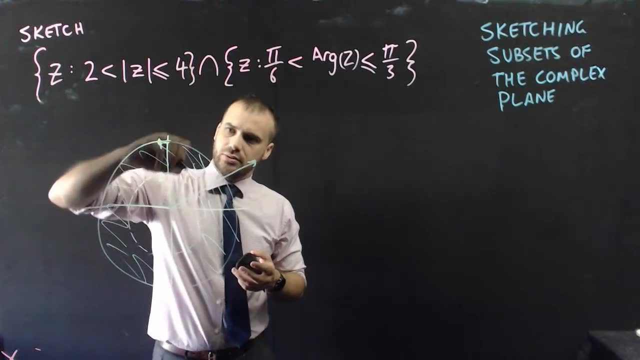 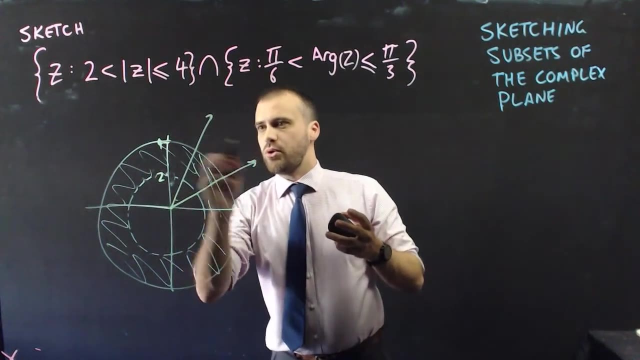 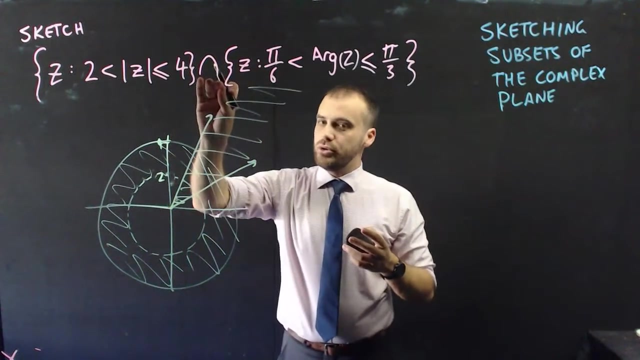 okay, pi on six is uh 30 degrees. uh, pi on three is 60 degrees. so now i can shade in. if i just consider this bit, i can shade in all of that right and shade in all of it. but i need both of these conditions to be met. so i'm not shading in all of it, i'm just shading. 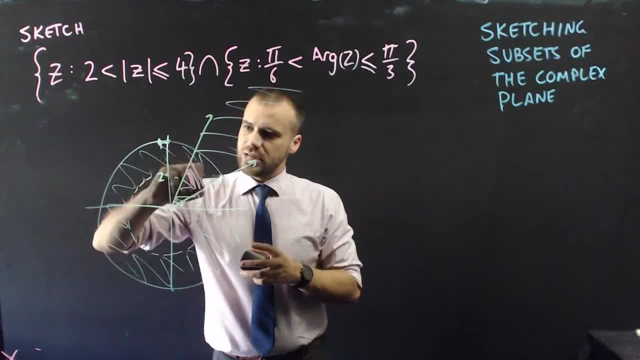 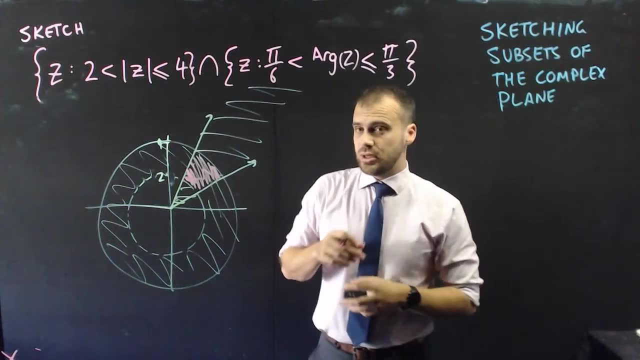 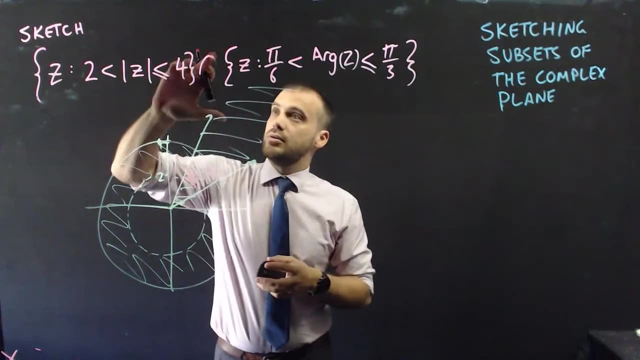 in the bit at which they overlap, which is this neat little bit, and i'm just shading in all of it and that's my answer to this question. now, perhaps an interesting question- and a question that i've already answered- is taking that and flipping it around like that. if i do that, i'm not saying that. 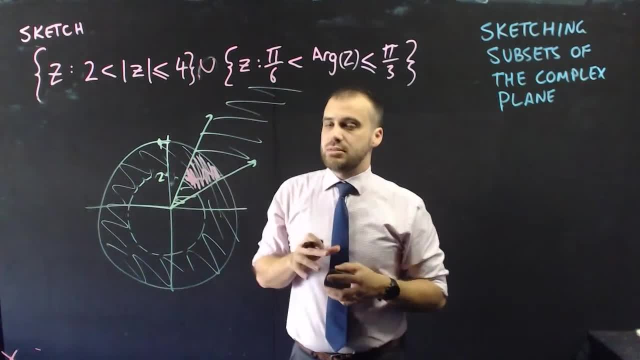 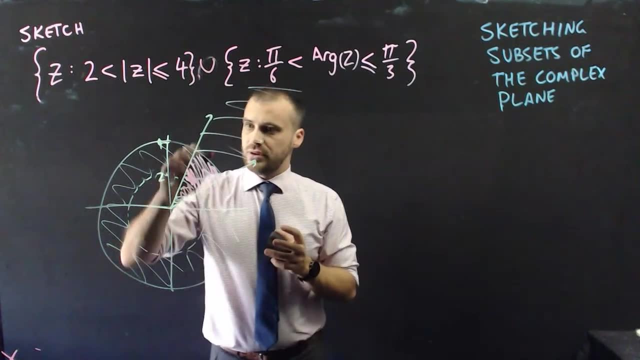 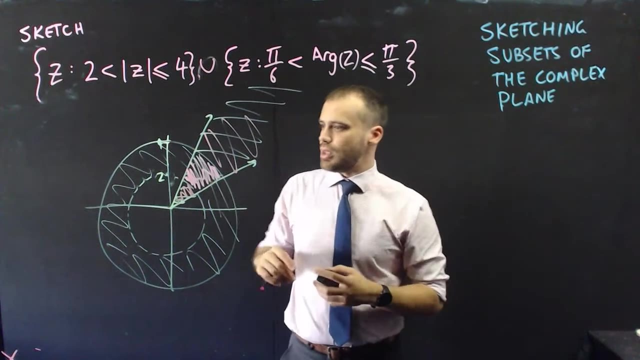 and that needs to be met. i'm saying that or that needs to be met, in which case everything i've shaded is valid. so this stuff is valid. so i'm just shading in all of it, and i'm just shading in all of it. this stuff and all of that stuff is valid because that is true, or that is true, okay. 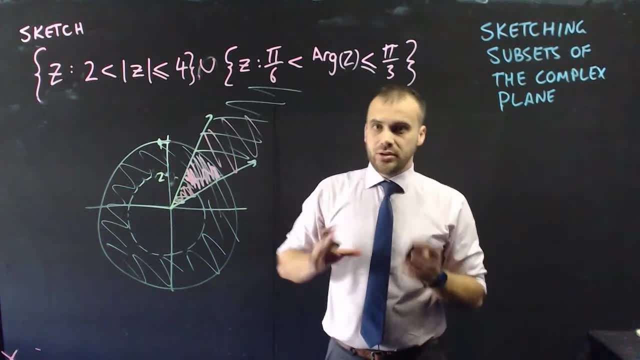 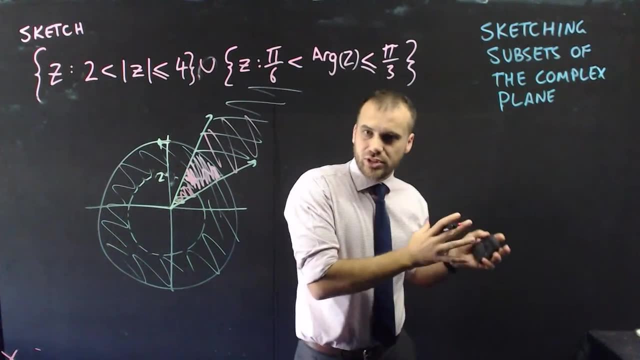 we've covered a lot of ground here again. practice these, but really try to understand what's being asked of you and then ask yourself: should i tackle this geometrically or should i tackle this algebraically?